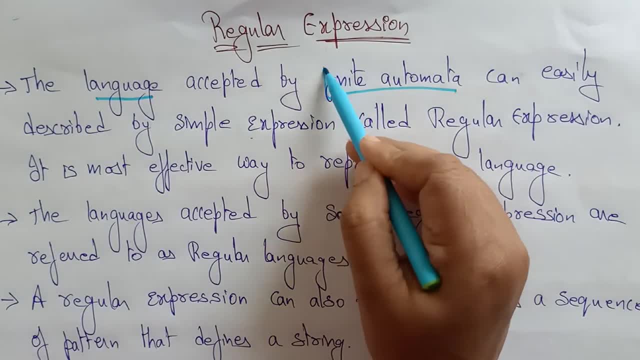 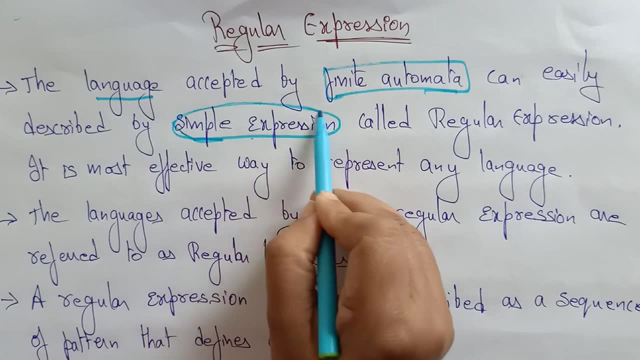 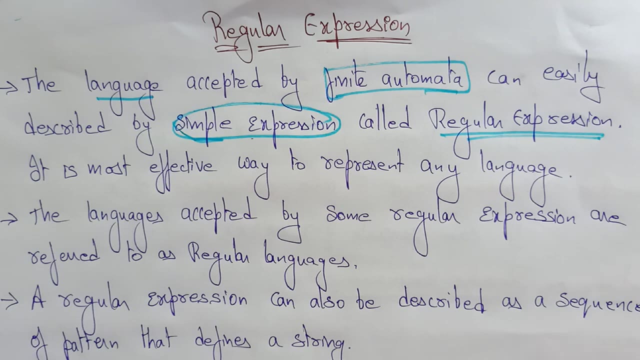 language you are taken. that language accepted by a finite automata can easily described by simple expressions. That simple expressions. you call it as a regular expressions. Okay, the language that is accepted by a finite automata can easily described by a simple expressions that we call it as a regular expressions. It is most effective way to 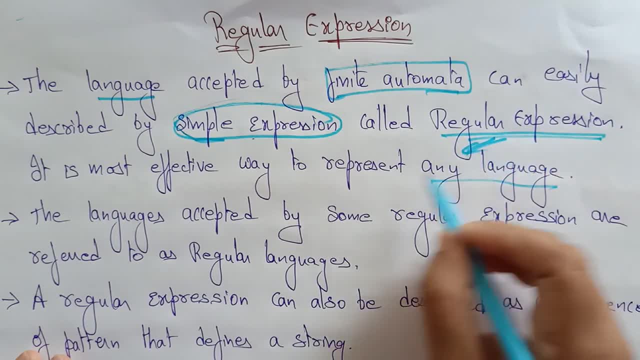 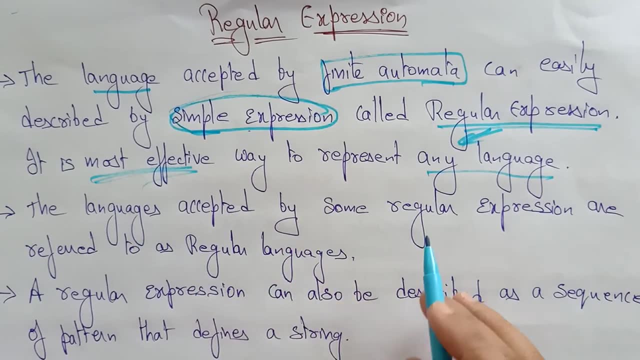 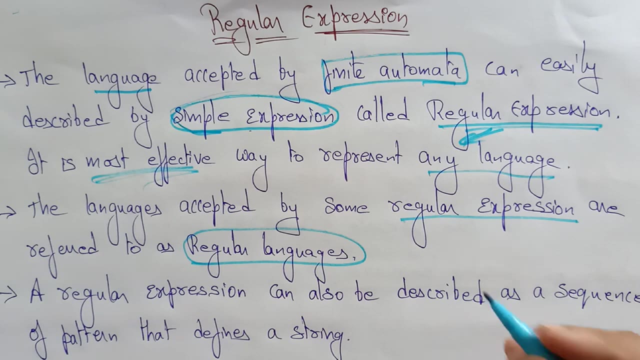 represent any language. So the regular expressions is a most effective way to represent any type of language. So the language accepted by some regular expressions can easily described by a simple expressions that we call it as a regular expressions. So whatever the language is accepted by regular expressions, so the language that is accepted 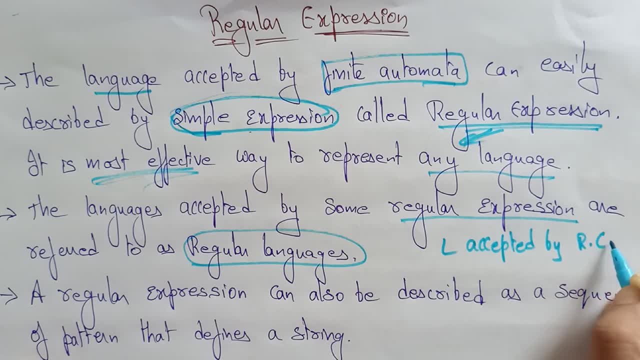 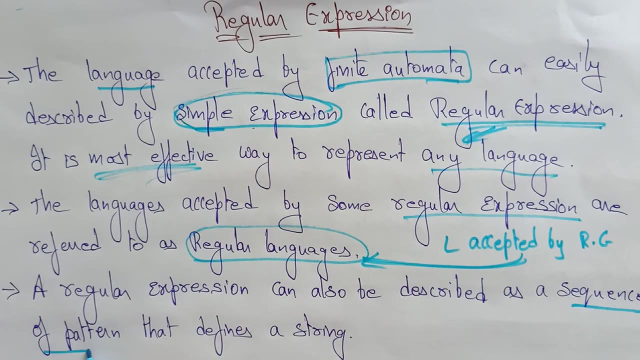 by regular expressions, we call it as a regular language. Okay, language accepted by regular expressions, we call it as a regular languages. A regular expressions can also be described as sequence of pattern that defines a string. An expression can also be described as a sequence. 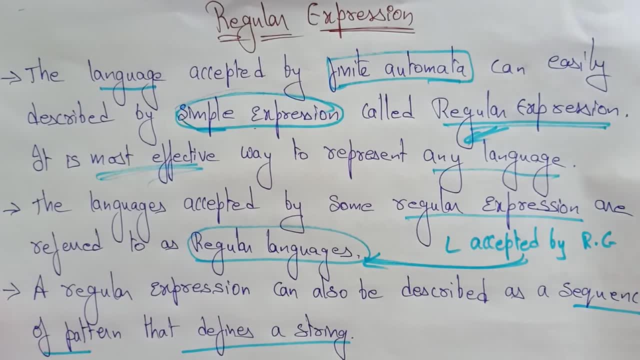 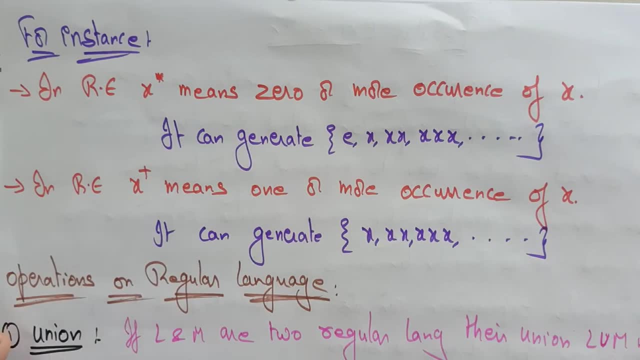 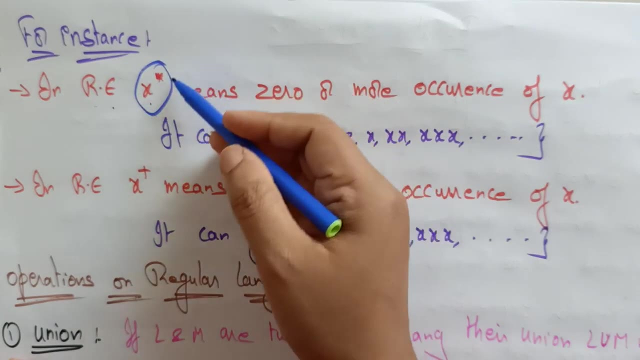 can be represented in the form of a sequence of patterns which defines the a string. that sequence of patterns, we call it as a string. So, for instance, let me take a regular expression that is x star. okay, x star. we call it as x closure. X closure means 0 or more occurrence of x. So 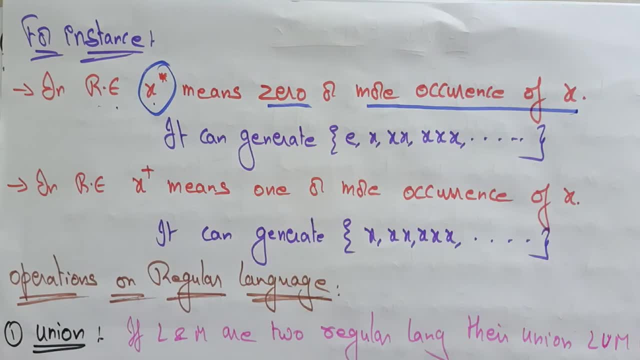 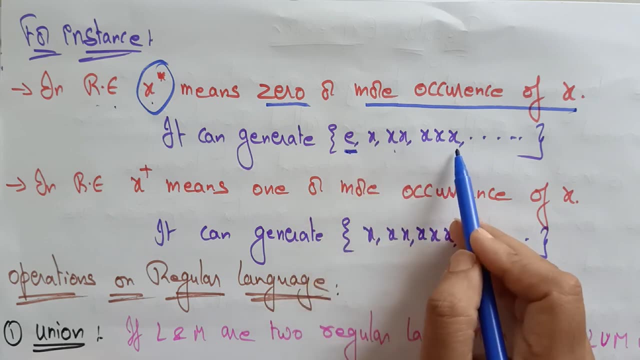 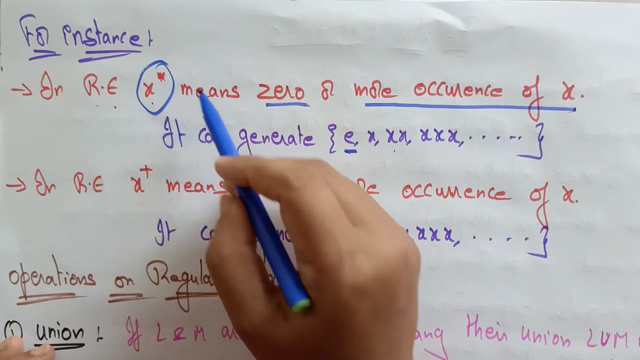 whenever you are seeing this x star or any language, any language with the star, it can be generated by the empty string that is the epsilon: x, x, x, x, x, x x, cube, x square, x, x, power 4, like that. So whenever you are seeing x power star, that is the x closure. there is a clean closure means. 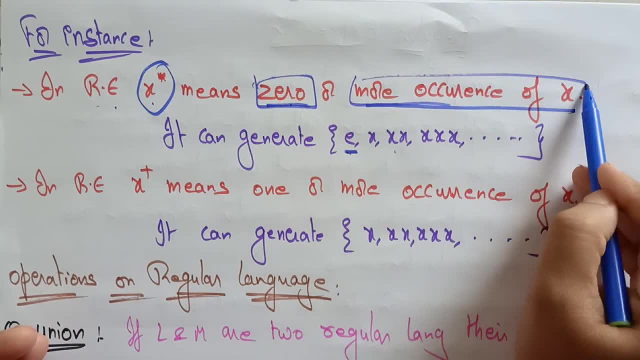 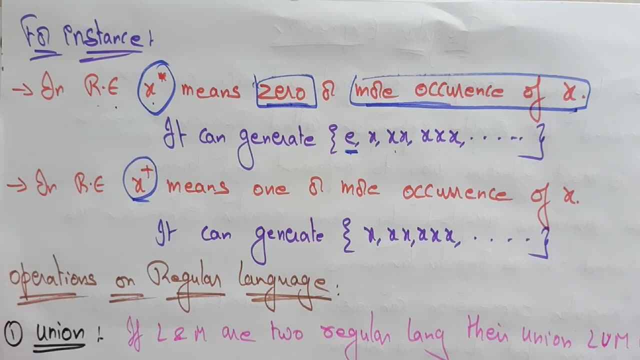 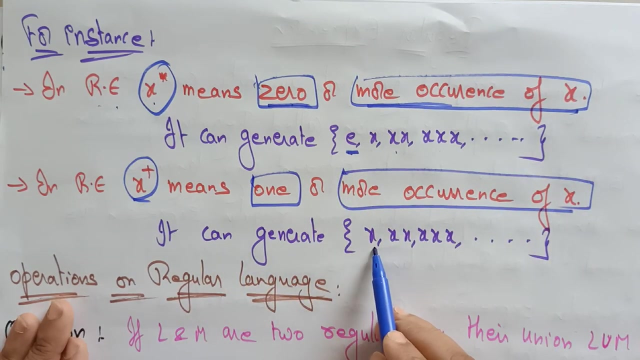 the 0, the 0 or more occurrence of x. Suppose, if you are seeing a regular expression with x plus x plus, this is x plus, which means one or more occurrence of x. So here the it can generate, it starts with x. it does not take the 0. okay, x plus does not take. 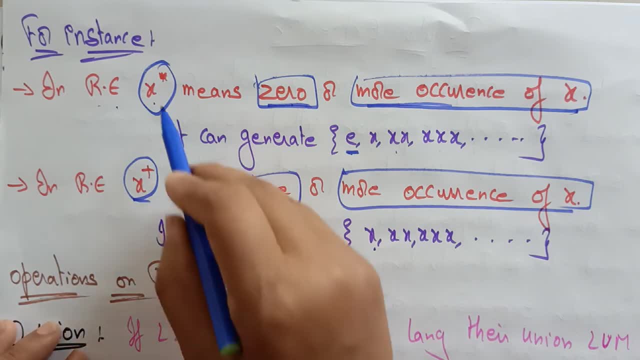 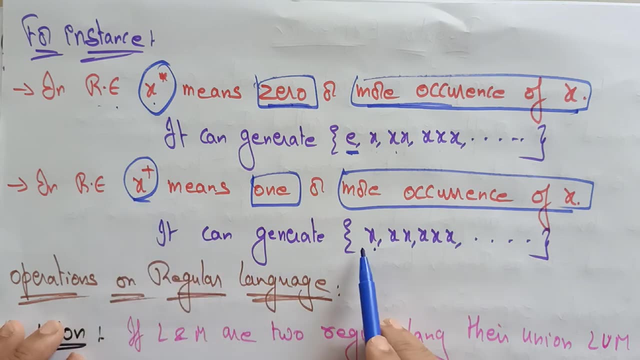 start does not start with 0, it starts with 1 only, but whereas x star, it starts with the 0. So that is why I have taken epsilon x x, x, whereas x plus means it starts with 1.. So you have to. 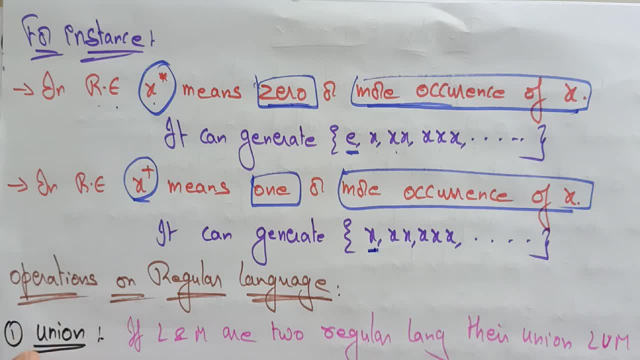 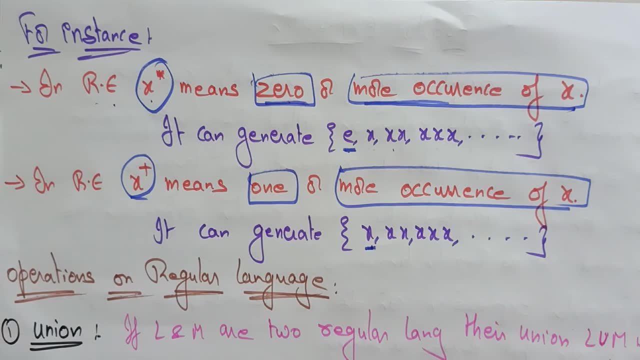 take starting x, do not take the epsilon which indicates the 0. So this is way you can represent the regular expressions. So let me explain The different operations on regular languages. So with the help of these operations you can easily construct the regular expressions, The operations on regular language. Suppose, if you 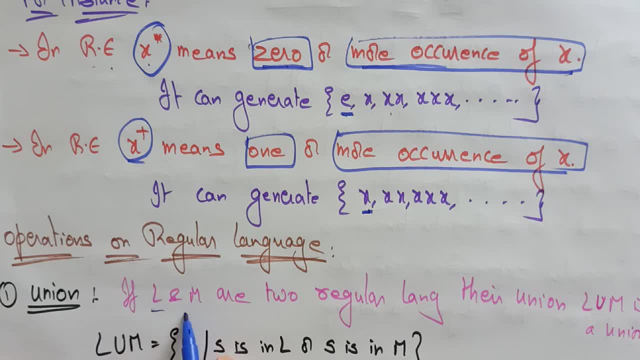 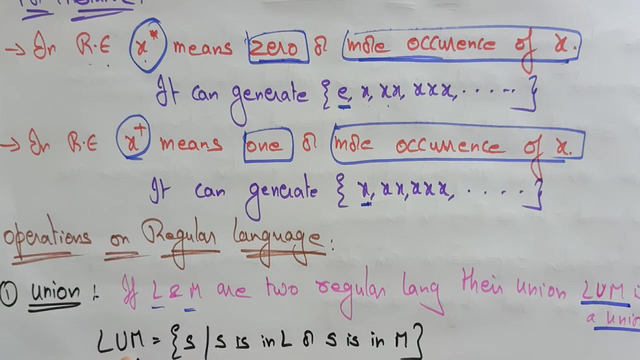 take two languages, that is a regular language- l and m- or two regular languages, their union. that is the sorry if language, two languages- l and m- are the same. So if you take two languages, l and m are two regular languages and their union is l union. m is also union. So here l union m. this is a two. 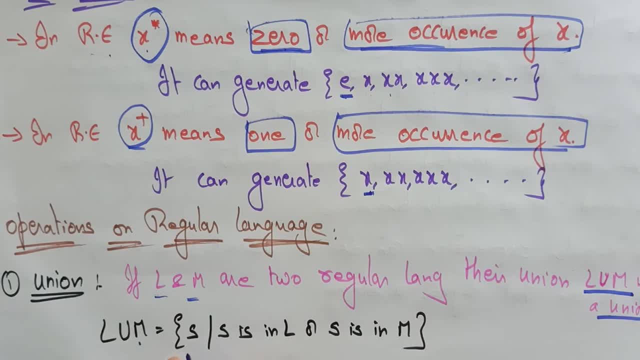 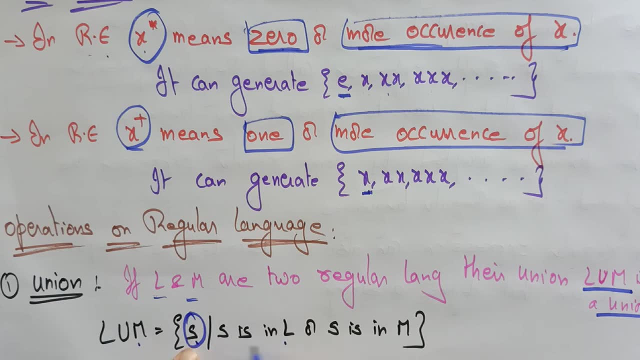 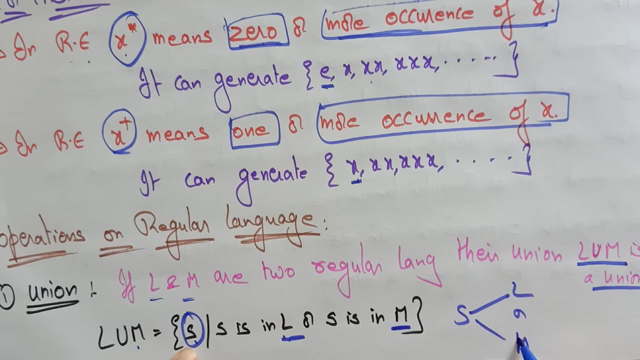 languages. l and m are two languages. this union is represents a string. okay, that string, that is, s, is in either in l or this string is either in present in m, So s is present in l or s is present in m. that is a union operation. 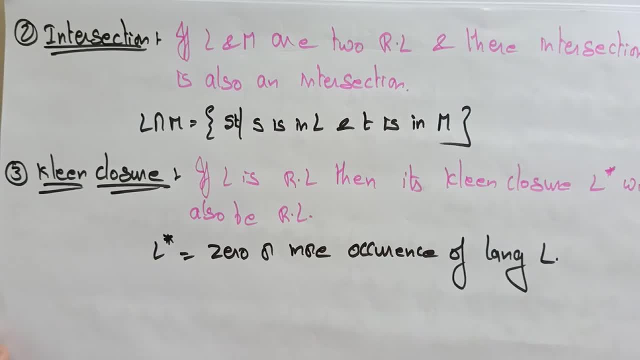 Next intersection. the another operation is an intersection. Suppose if two languages, that is, l and m, or two regular languages and their intersection is also an intersection, that is this, can be represented. that is l intersection m. So here l intersection m we are getting. 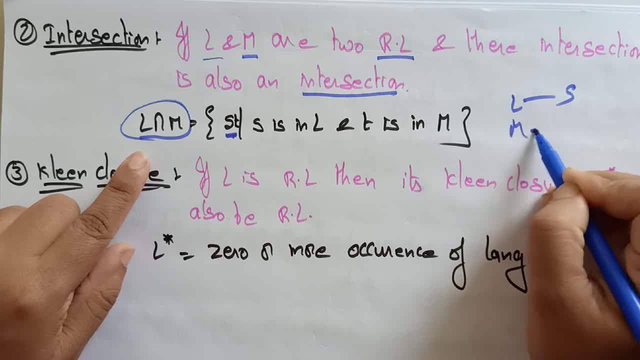 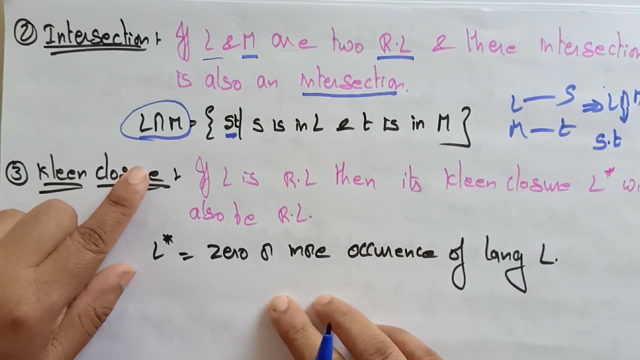 two strings: l consisting of s and m consisting of t. whenever you are taken l intersection m, It multiplies S into T, where S is in L language and T is in M language. okay, S is in L language and T is in M language. 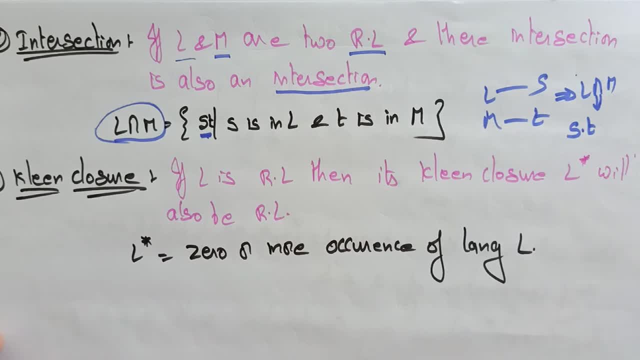 Next is a clean closure. Another property is a clean closure. The clean closure: if L is in regular language, okay, Whatever the L language that we have taken that is in regular language, Then its clean closure- that is a L star- will also be regular language. 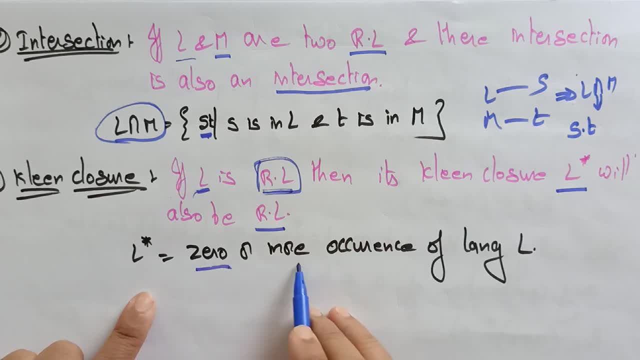 So L star is represented as it's a zero or more occurrence of languages L, So that L star will start with the zero or more languages of L, Whatever the language, that is string consisting of that strings. you can be placed A plus B A into B A plus B star, like that, anything, okay.